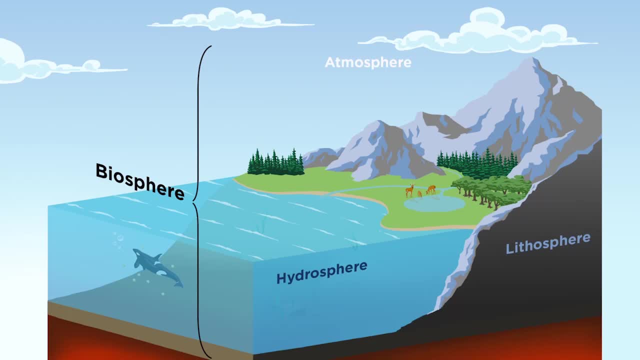 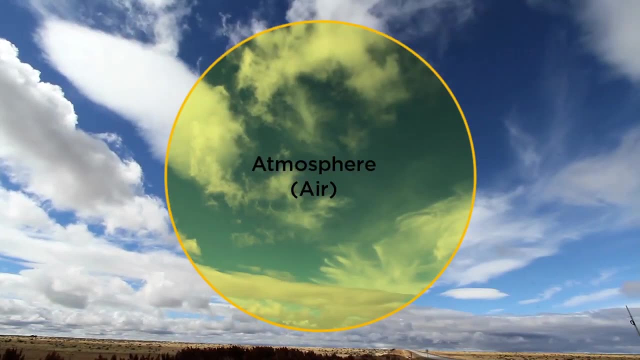 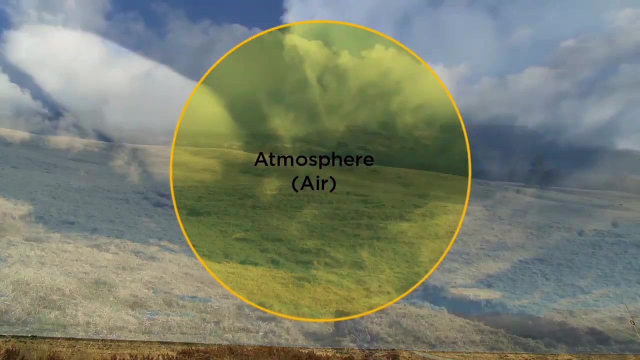 these systems. we need to understand that each system is a group of related elements that form a complex whole. Take a breath. You are breathing in air from our atmosphere. The atmosphere, from the Greek word atmos, meaning vapor, is a thin layer of gas. 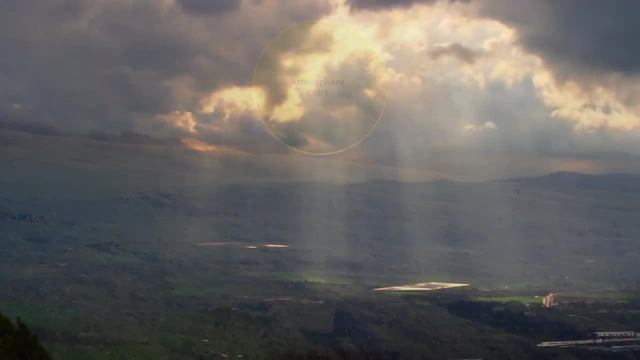 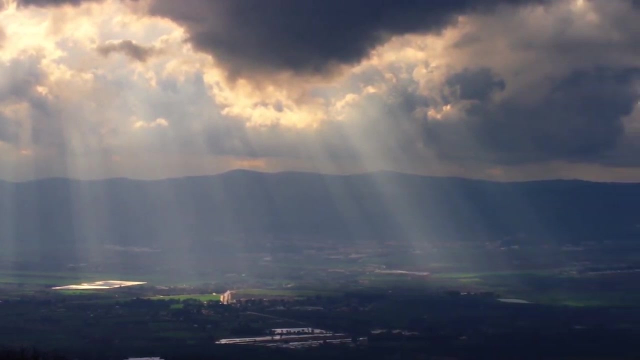 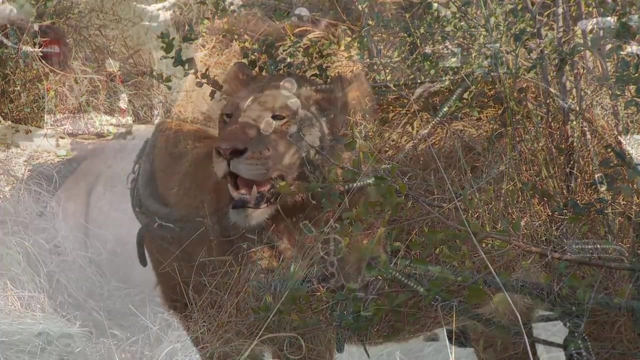 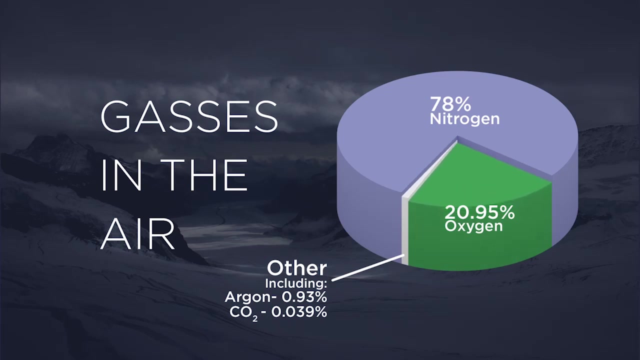 surrounding the planet. The atmosphere serves many functions: It offers protection from UV radiation, helps hold in heat to warm the planet's surface and contains the oxygen and carbon dioxide required for animal and plant life. Earth's atmosphere comprises 78% of nitrogen- 20.95%. 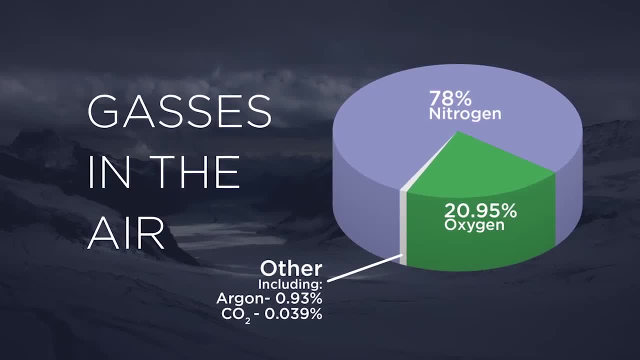 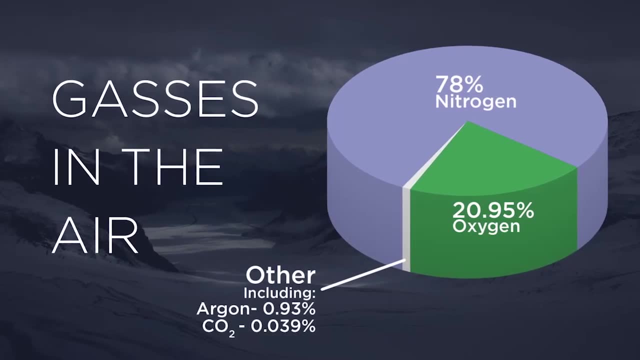 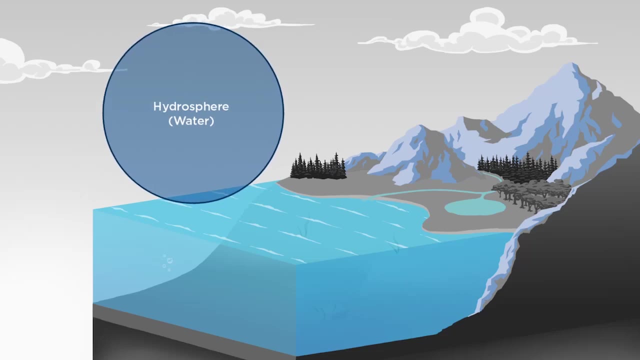 of oxygen, 0.5% of oxygen and 100.5% of hydrogen. Its atmosphere is also composed of three multiple 0.93% of argon and 0.039% of carbon dioxide and other gases. The hydrosphere, from the Greek word hydro, meaning water, includes all of the water covering. 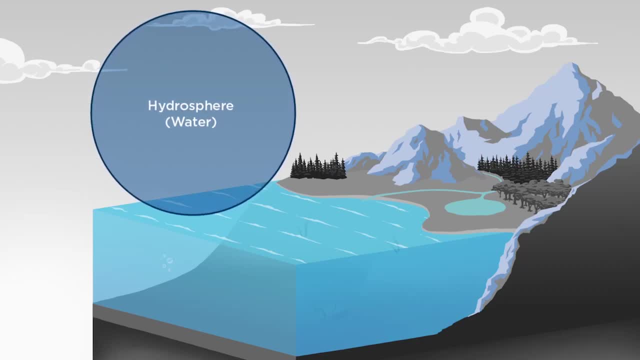 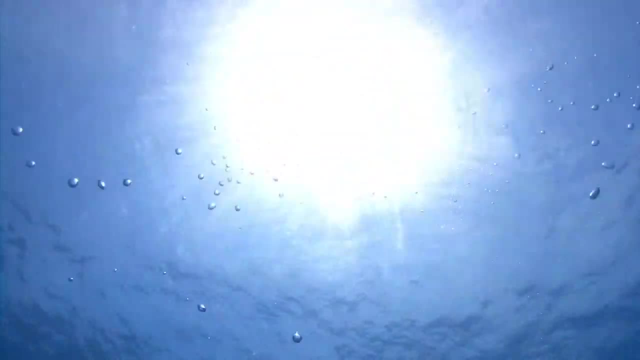 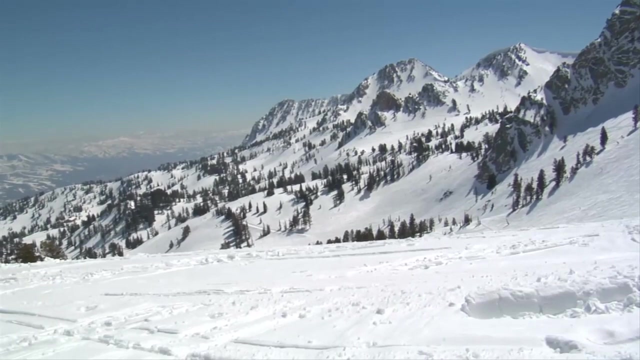 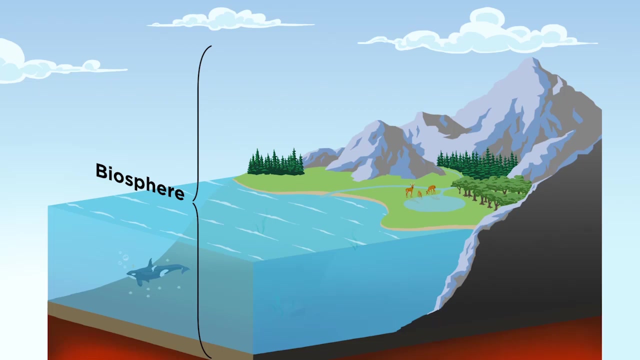 Earth, both in liquid and solid form. 71% of Earth is covered in water. From the depths of the ocean to the ice-capped peaks of the mountains, the hydrosphere is all around us. Our biosphere- bio meaning life- contains all of the life on Earth. 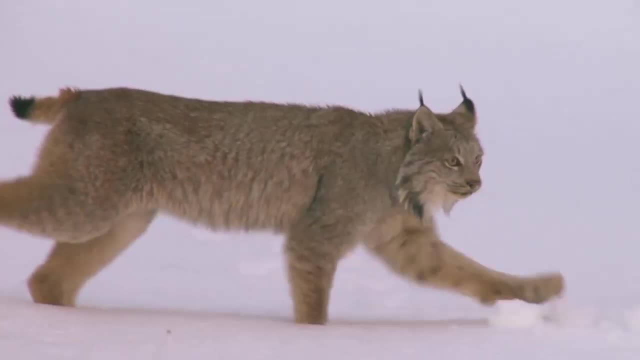 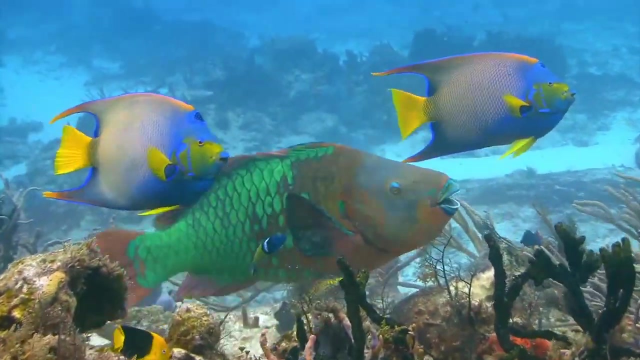 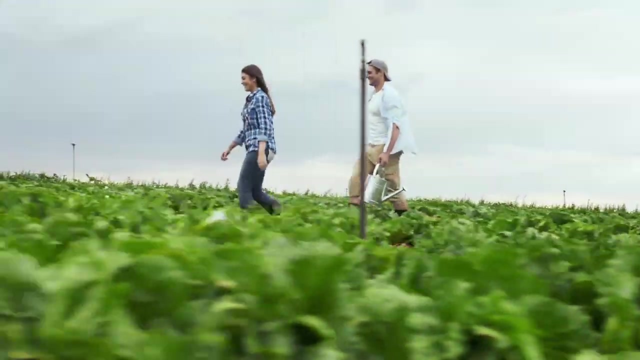 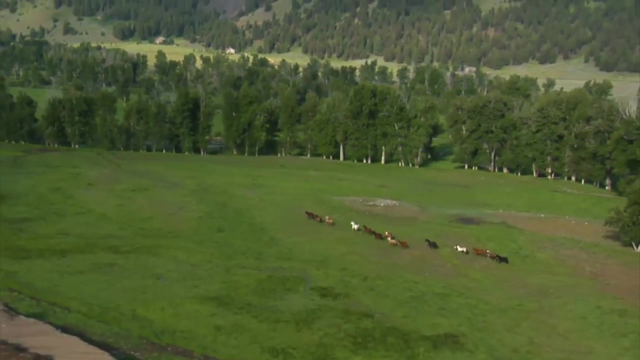 Living beings are found everywhere on Earth, even on the parts that appear to be uninhabited. The biosphere overlaps the atmosphere. We are part of the biosphere, as are the crops that we grow and the pets that we keep. Every living being, from tiny bacteria to blue whales, is part of Earth's biosphere. 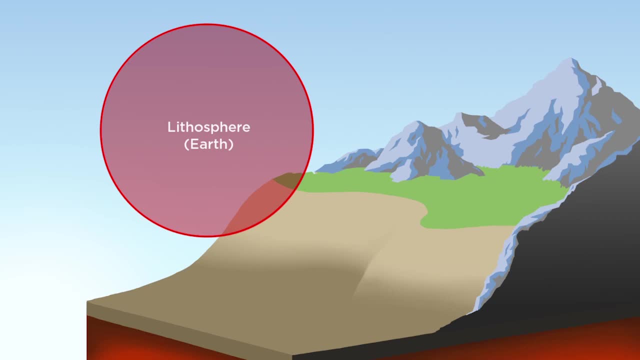 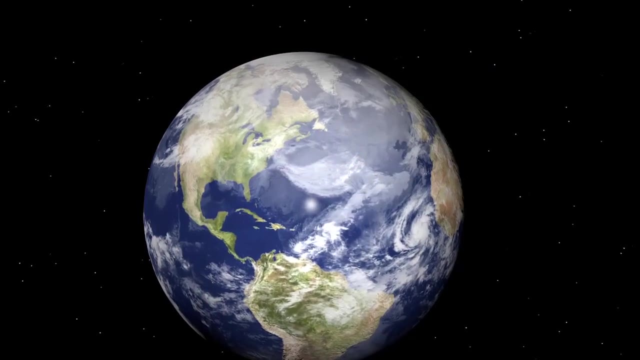 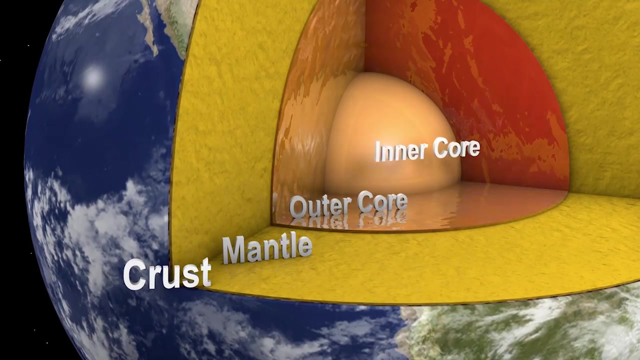 Earth's crest and upper part of the mantle make up the lithosphere, which is from the Greek word for stone, lithosphere. Our lithosphere consists of approximately the first 60 miles of solid material from the surface of the planet down. This is also referred to as Earth's crust.